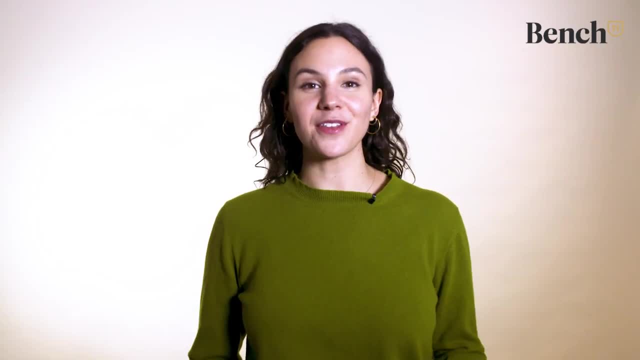 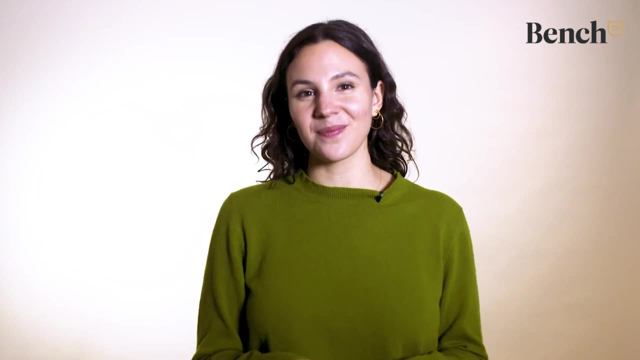 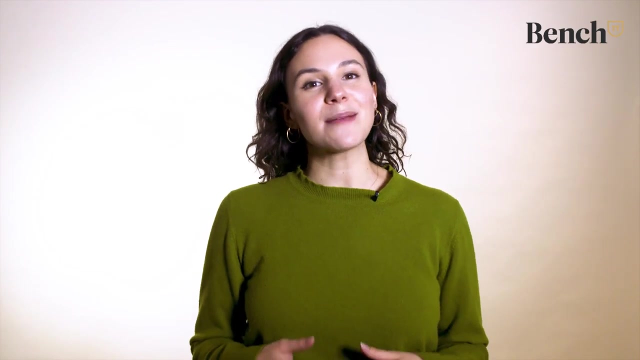 picture of your company's financial health. If you need a template for the balance sheet, income statement and cash flow statement, you can find links to those in the description below. Let's start with the balance sheet. A balance sheet is a snapshot of your business. 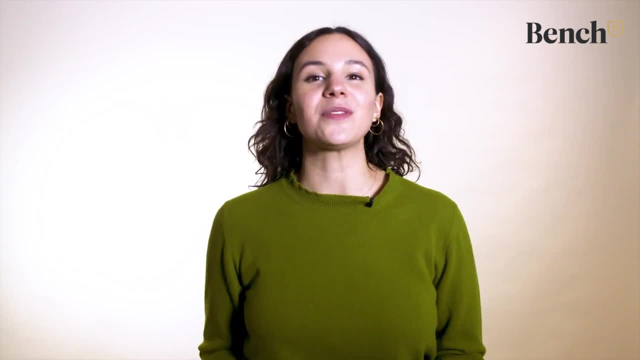 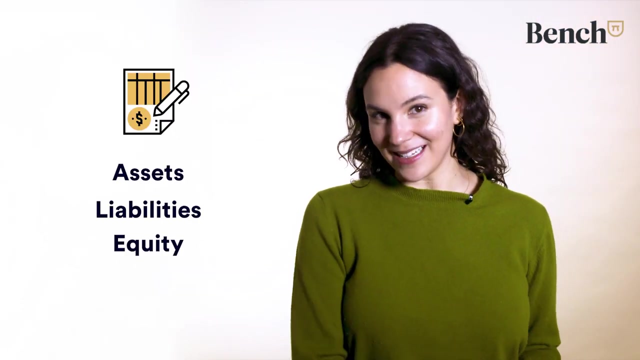 finances. as it currently stands, It tells you about the assets you own and liabilities, aka debts that you owe at a particular point in time. Balance sheets are broken up into three general categories: Assets, liabilities and equity. Here's what it looks like. This one happens to be the 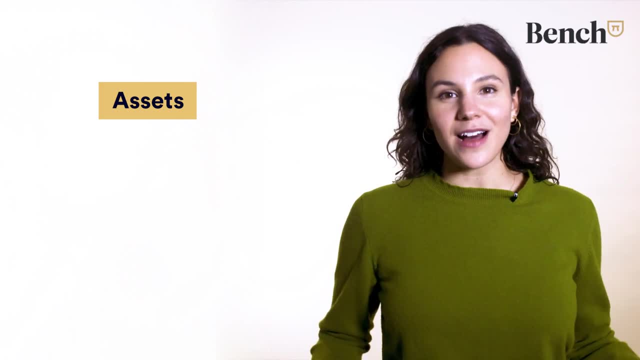 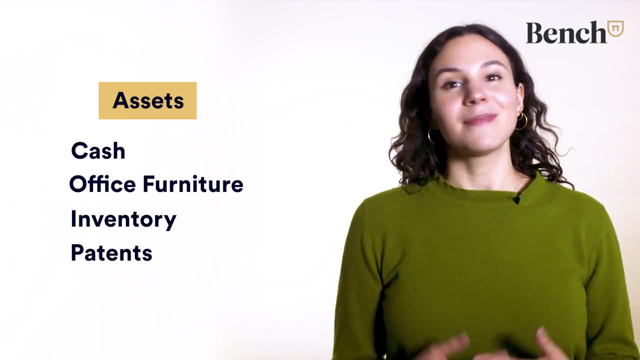 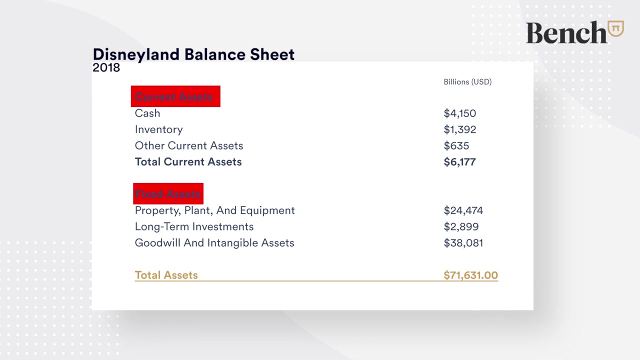 balance sheet for Disneyland. Assets are anything valuable that your business owns, including cash, office furniture, inventory, patents, etc. Sometimes they're broken up into current assets and fixed assets, like you see here. Current just means it's cash or cash equivalent, something you 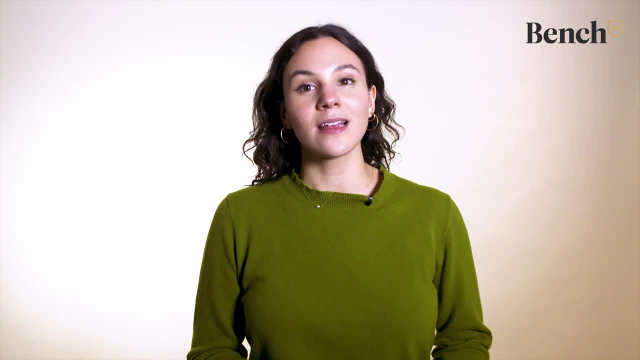 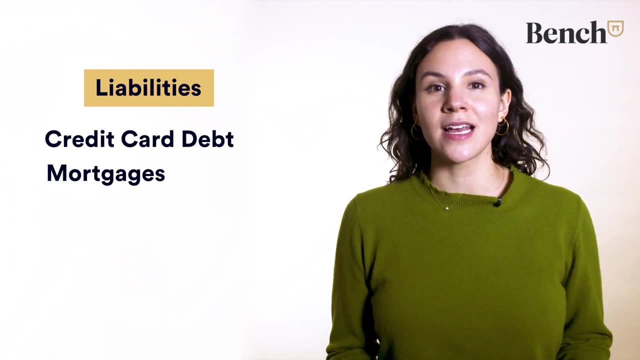 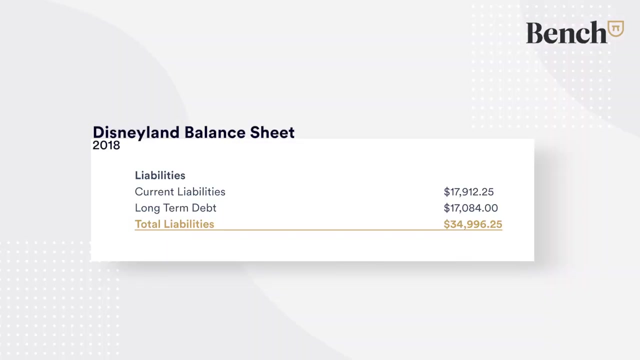 can sell quickly. Next, we have liabilities. Liabilities are debts you owe to other people. These can be things like credit card debt, mortgages and accrued expenses such as utilities, taxes, etc. Or wages owed to employees. Like assets, they're normally split into current liabilities that you 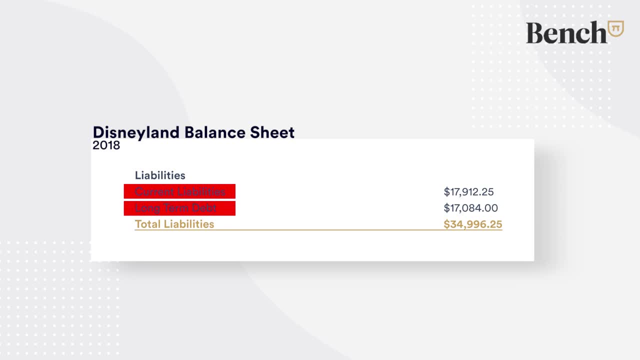 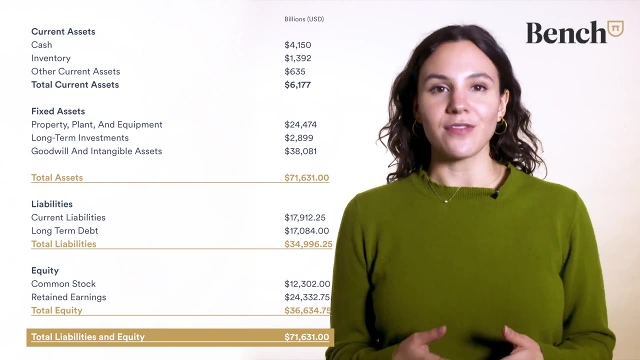 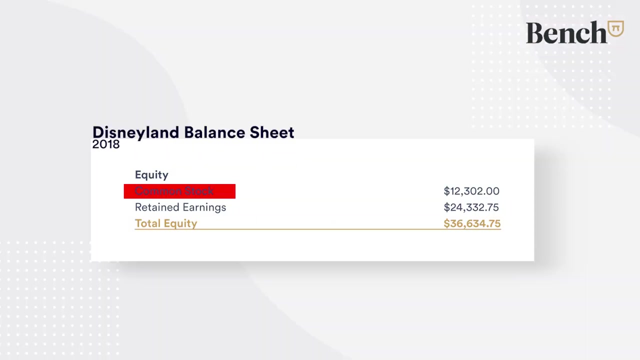 owe within the next 12 months and long-term debt beyond 12 months. The last category is equity. Equity is the remaining value of the company after subtracting liabilities from assets. Equity can come in the form of common stocks, like when you buy stock in a company like Apple, or in the form 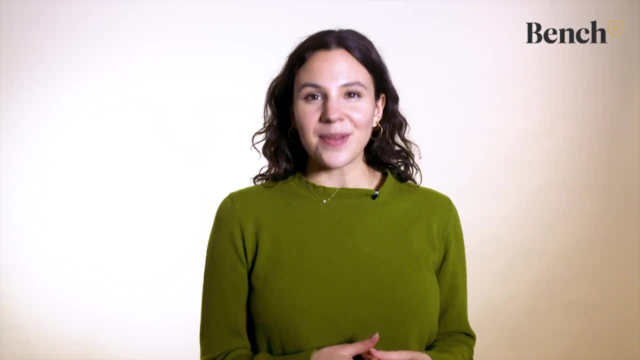 of retained earnings. And yet, the more liabilities you have, the more liabilities you have to pay off. When you pay off shares of shares, you're still only putting in money. And what kind of balance sheet do you actually have? As you can see, I have a lot ofhn the balance sheet in this section. 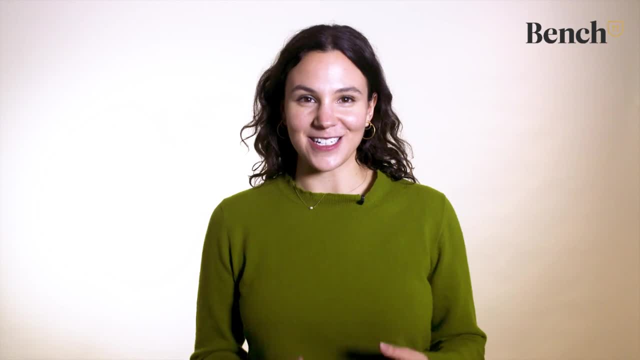 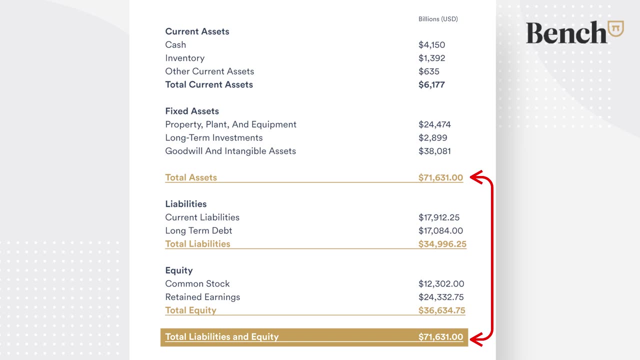 The balance sheet will add up the amount of net income left over for your business after you've paid out any dividends to shareholders. Now here's where the whole balance part of the balance sheet comes in. The value of the assets section will always balance with the liabilities and equity section. 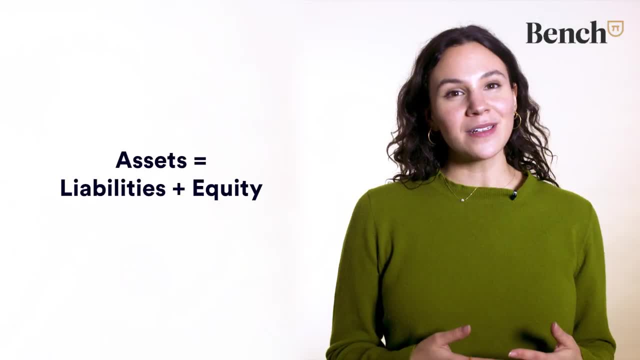 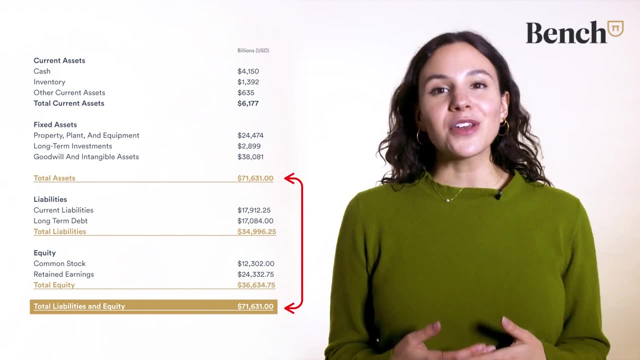 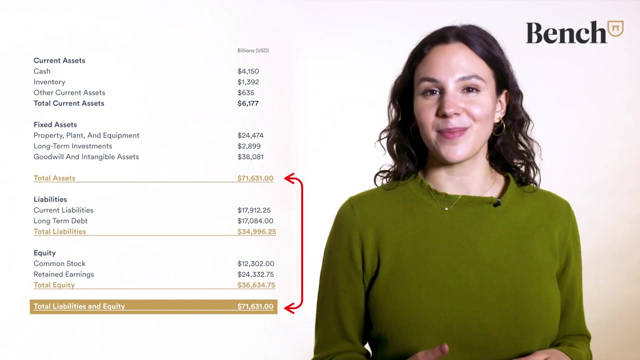 That's the balance sheet equation: Assets equal liabilities plus equity. So you can see on the Disneyland balance sheet that these three things are conduct for the balance sheet equation. The value of the assets is the exact same as the liabilities plus equity. That's how you know they prepared the balance sheet right. 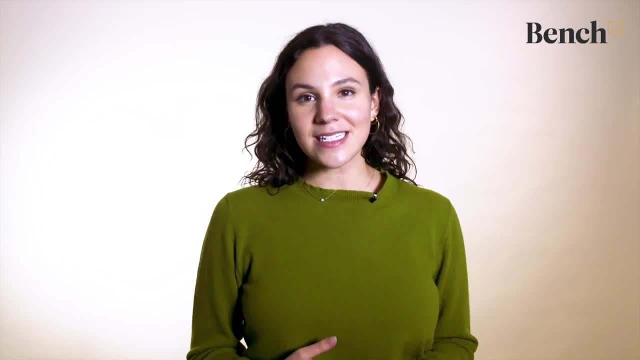 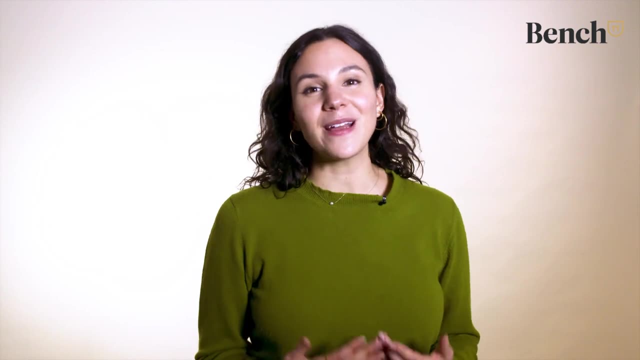 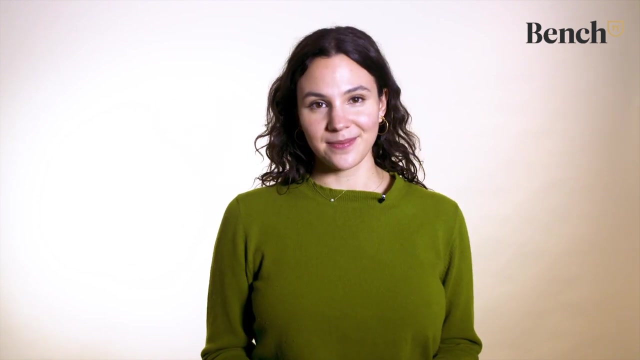 That's a quick overview of the balance sheet. Big businesses, like banks, prepare a balance sheet every day. Small businesses, like a brand new Etsy shop, might only prepare a balance sheet every three months. It all depends on how many assets are moving in and out of your business. 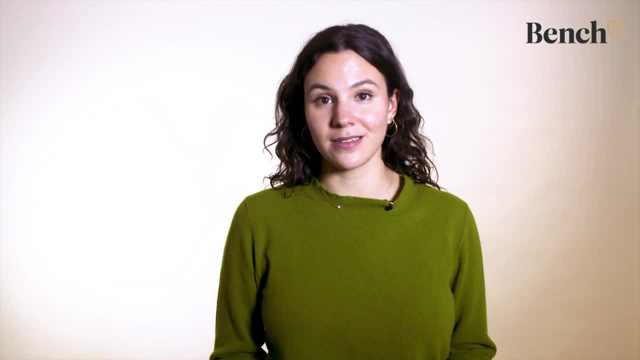 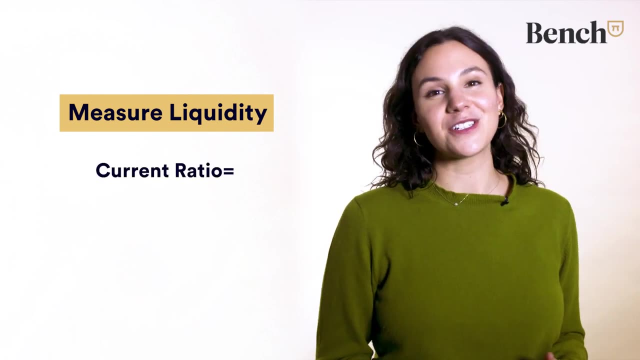 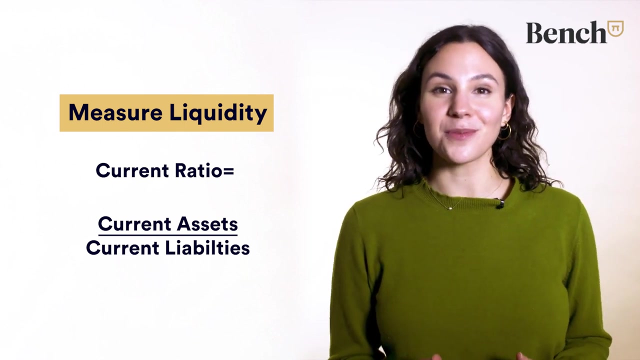 Now, what can you really learn from a balance sheet? Tons of things. For one, you can measure the liquidity of your business with the current ratio, which is current assets divided by current liabilities. This tells you if you'll be able to pay off your debts in the next 12 months. 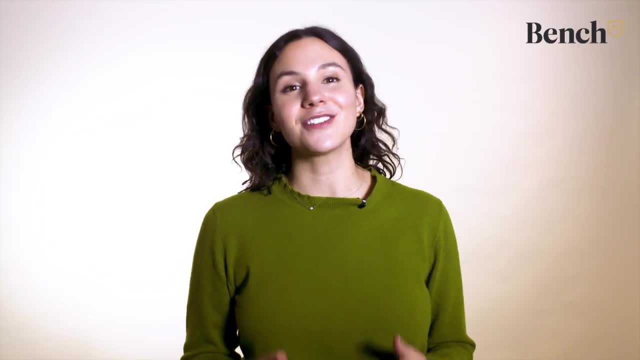 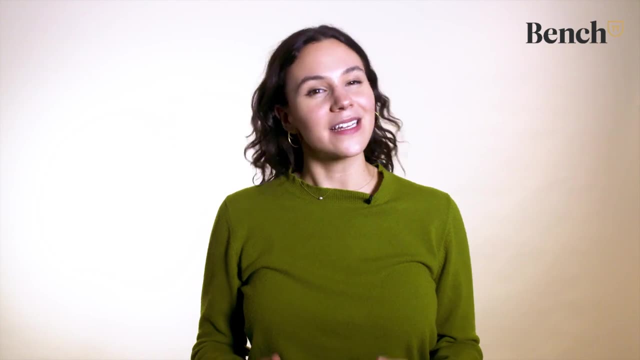 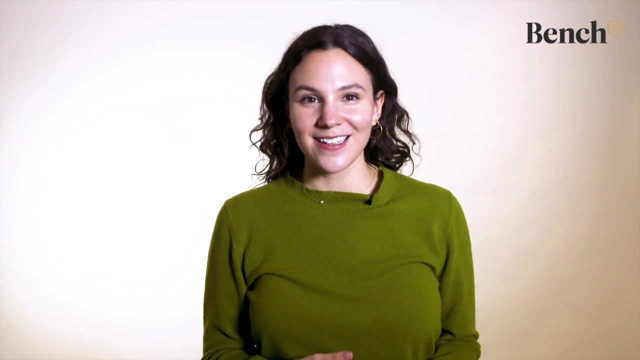 And there's lots of other useful ratios you can calculate using just your balance sheet. Next, let's talk about the income statement. The income statement is the balance sheet. The income statement tells you how much money your business has spent and how much it has earned in a specific period. 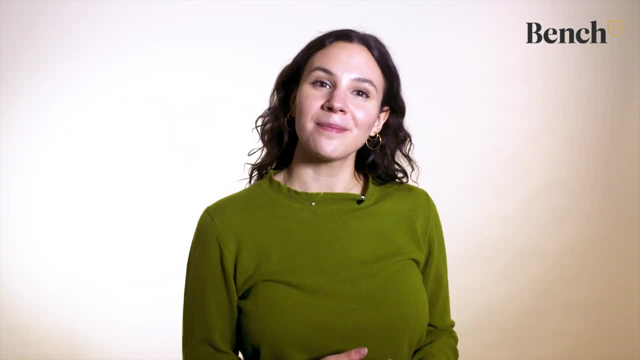 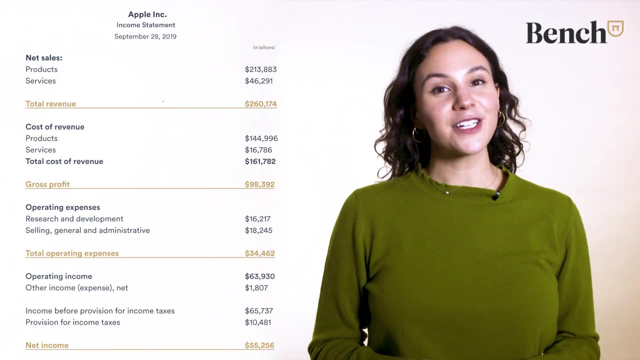 That lets you calculate your net profit, otherwise known as your bottom line. The reason it's called the bottom line is because net profit is at the bottom of your income statement. Here's what an income statement looks like. This one is from Apple. 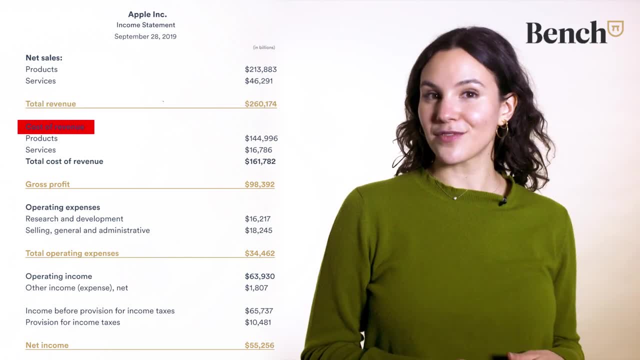 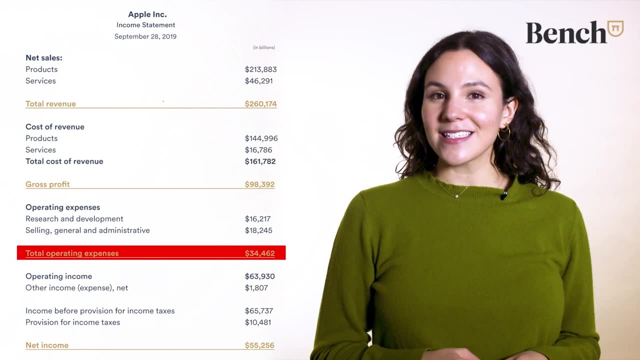 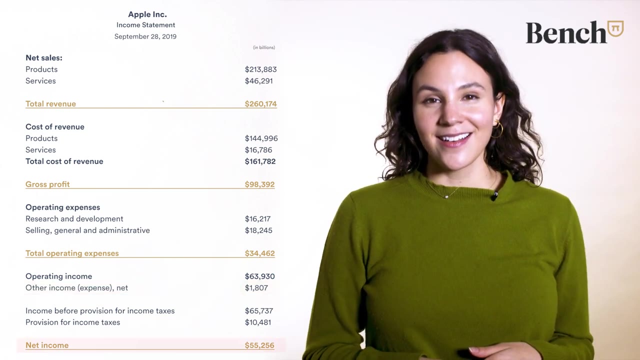 It has six main sections: Revenue, cost of revenue, gross profit minus cost of revenue, operating expenses, operating income or loss taxes and other non-operating expenses. and net income. Let's go through what each section means. We'll make it quick. 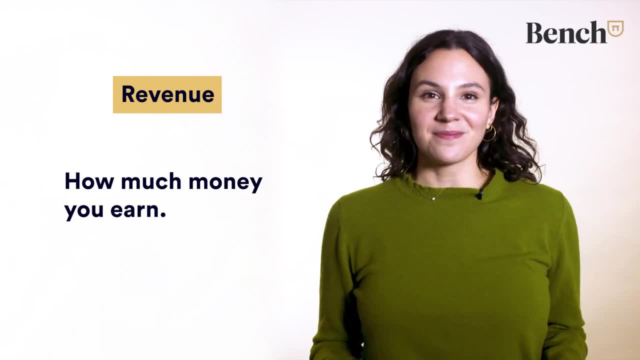 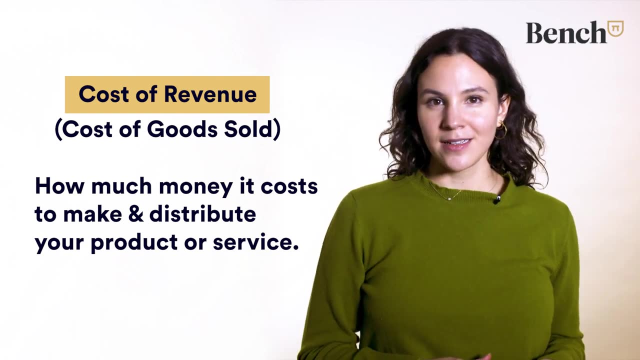 Revenue is how much money you earn. Pretty basic Cost of revenue or cost of goods sold is how much money it costs to make and distribute your product or service. This doesn't include things like the cost of your bookkeeper or the cost of rent. 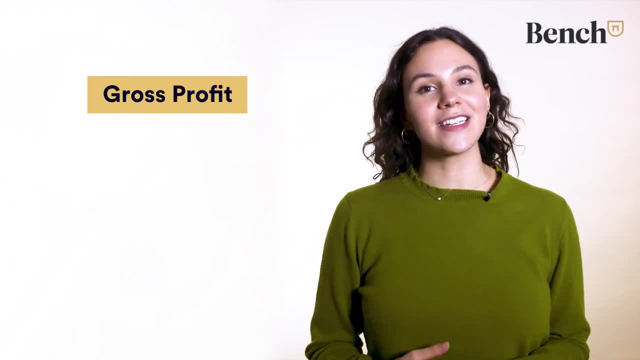 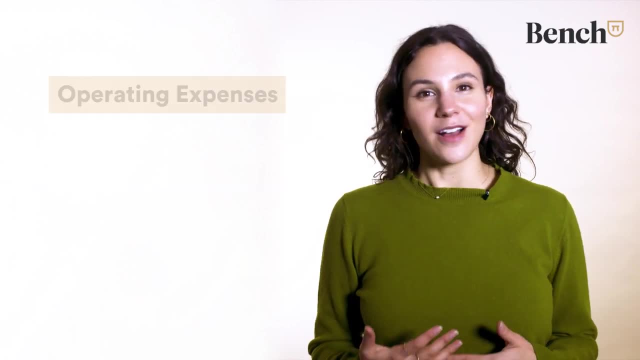 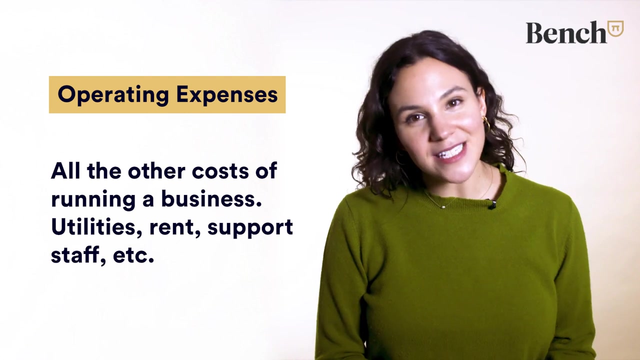 Those are operating costs. Gross profit is your revenue minus cost of revenue, Essentially how profitable your products and services are. Operating expenses are all the other costs of running a business: Utilities, rent, support staff who aren't making or distributing your products, etc. 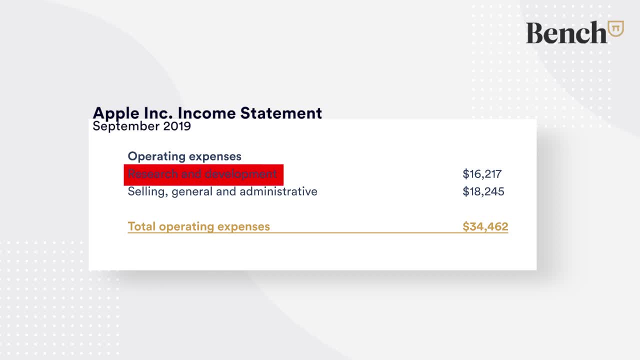 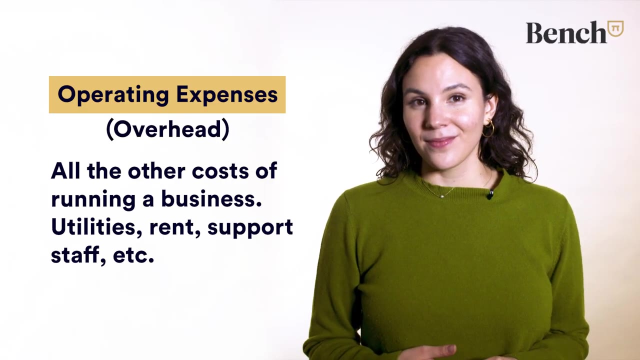 You can see for Apple. they also include research and development here, Since the R&D team isn't exactly making products, They're just doing research that may or may not lead to a new product. Operating expenses are also known as overhead. Operating income or loss is your gross profit minus operating expenses. 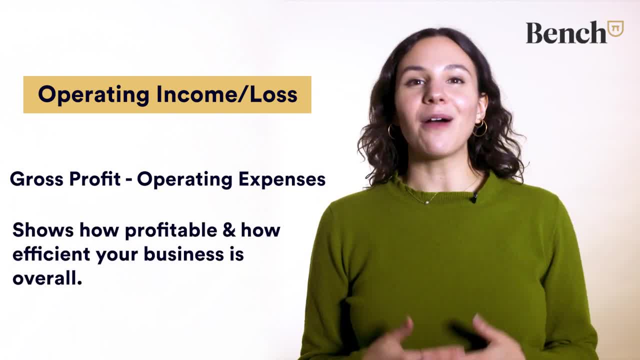 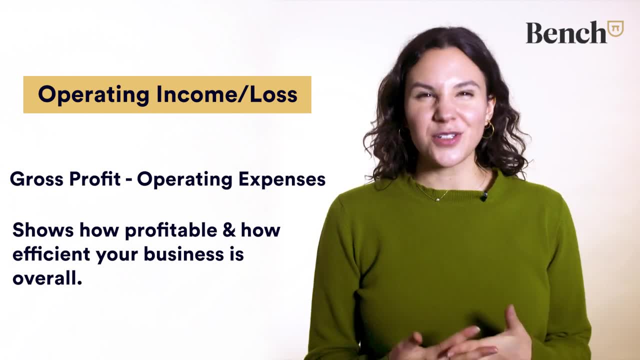 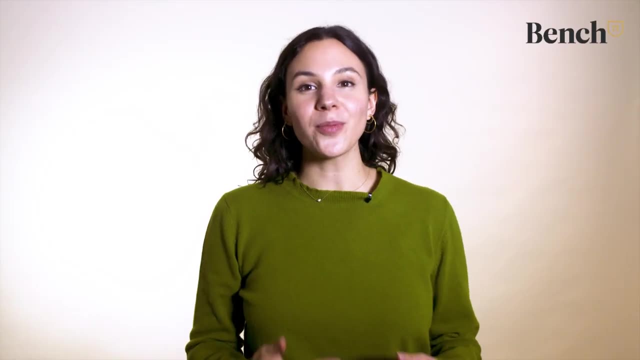 This shows you how profitable your whole business is, how efficient your business is at making money. You might have a nice gross profit but you spend way too much on rent and office snacks. So overall you're losing money. After you calculate your operating income or loss. 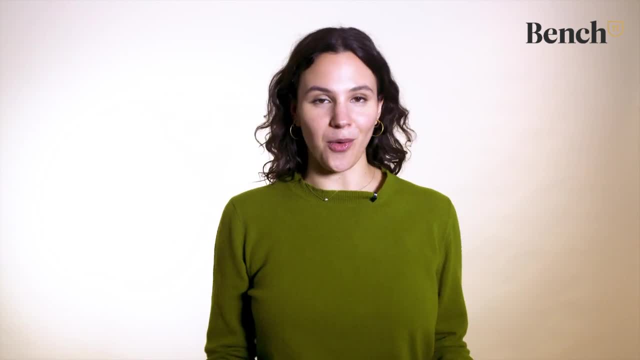 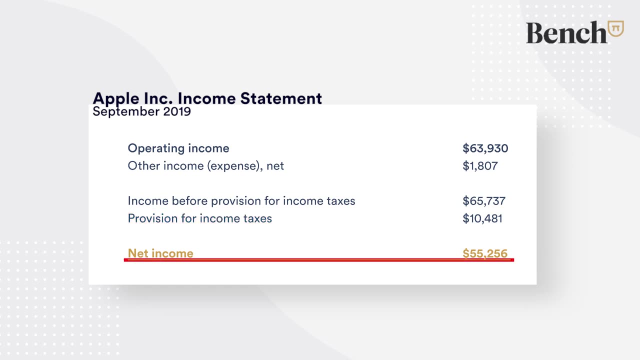 you need to take into account things that are somewhat out of your control, mainly taxes. After you've subtracted taxes from your operating income or loss, you get the bottom line, your net income. That's how much money you walk away with after you've subtracted everything else. 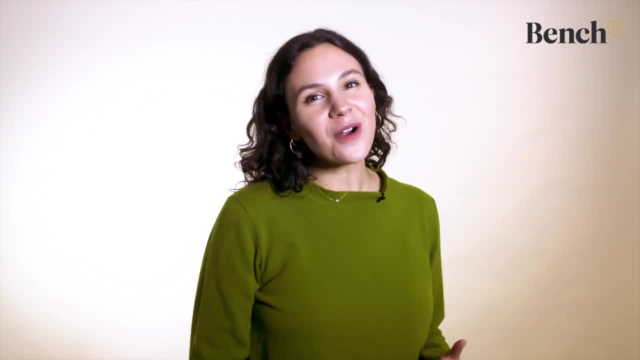 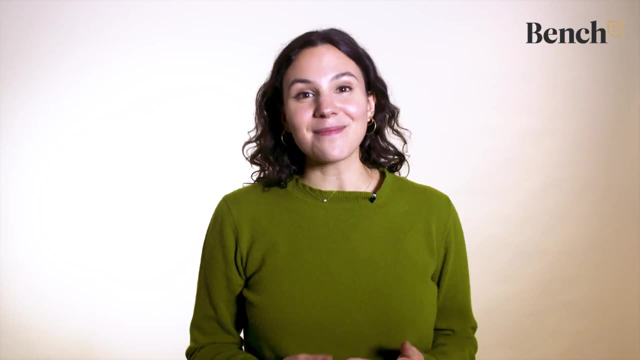 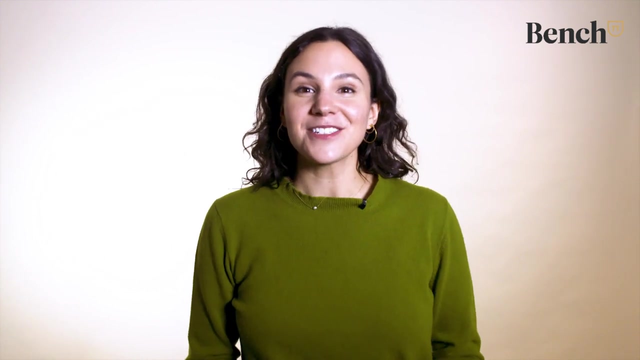 The value of the income statement is a little more obvious to most people compared to, say, the value of the balance sheet. It shows you if you're making money, if your business is profitable or not. That is super useful. More than that, it shows you if you're spending too much money producing your products. 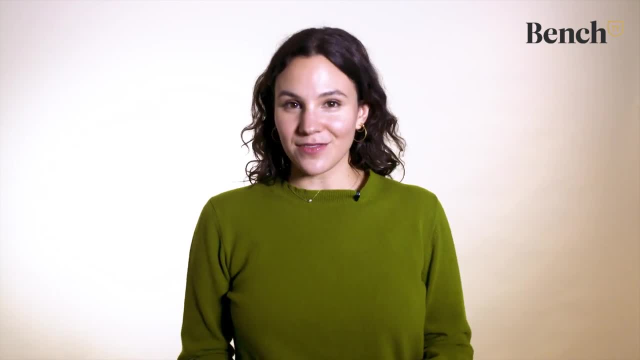 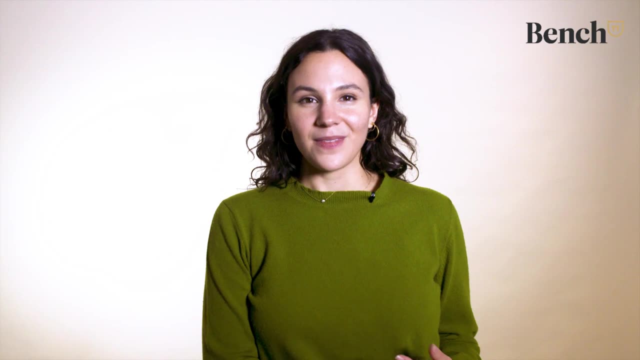 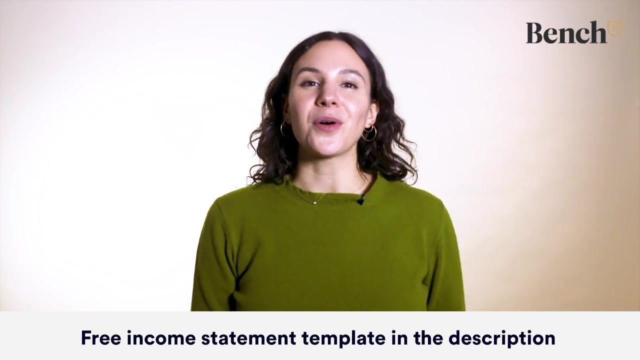 or if you're spending too much money on overhead, the cost of running your business. more generally, You'll want to consult your income statement regularly. If you want an income statement of your own, you can click the link in the description where you'll find a simple income statement template of your own. 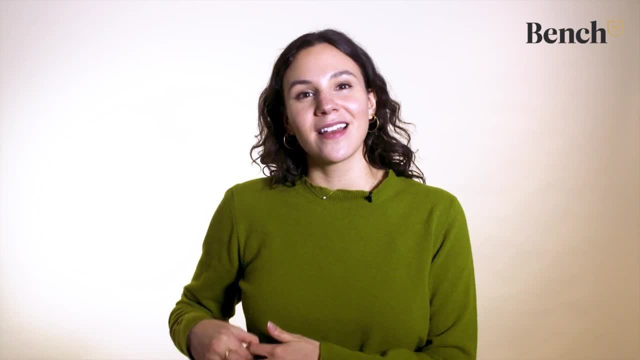 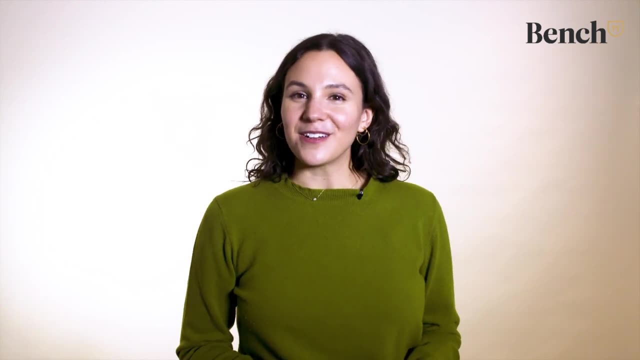 created by our expert bookkeepers here at Bench. If you don't want to do your own bookkeeping and make your own income statements, you can check out Bench. We'll do your bookkeeping for you and send you an income statement every month. 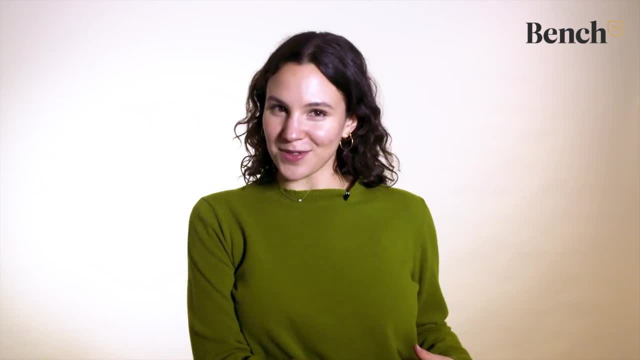 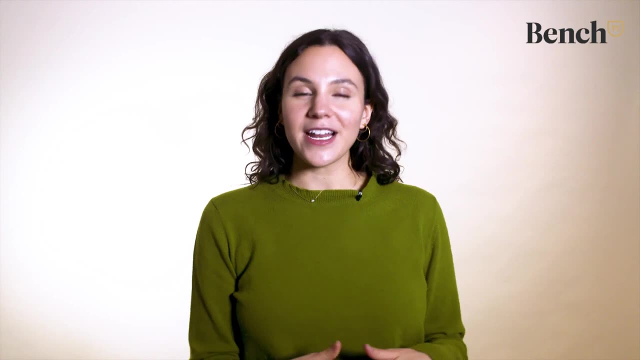 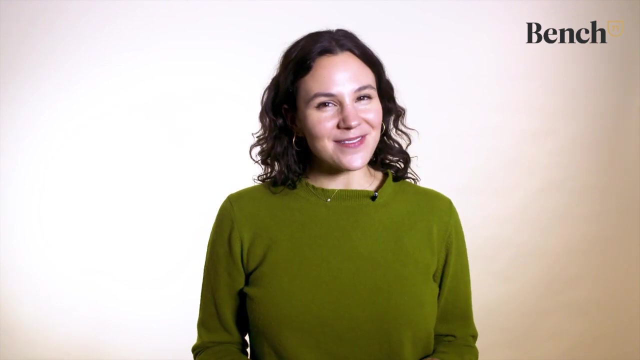 Anyway, on to the last financial statement, your cash flow statement. The cash flow statement tells you how much cash entered and left your business over a particular time period. You might ask: isn't that the same as the income statement? No, The income statement shows you how much you spent. 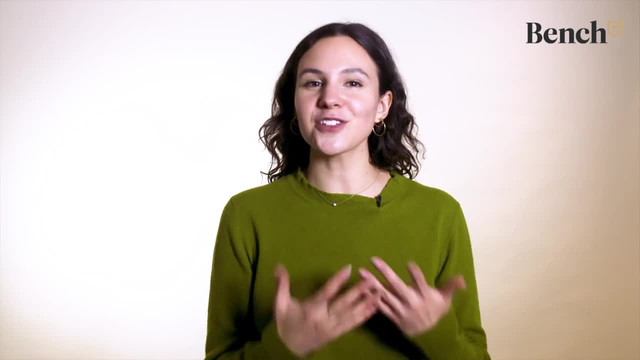 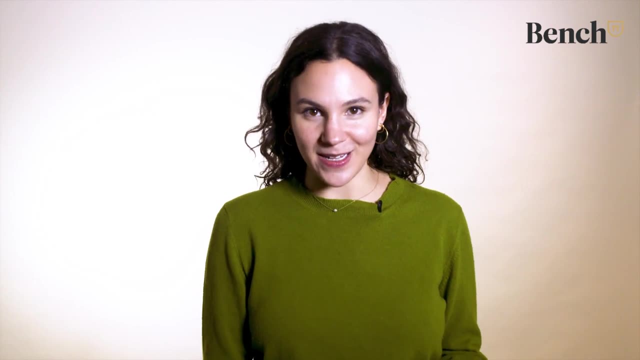 and how much you made. The cash flow statements show you what the cash reality of your business is. This is most relevant for businesses that use the accrual basis of accounting. Let's say, your income statement says that you made $10,000 in March. 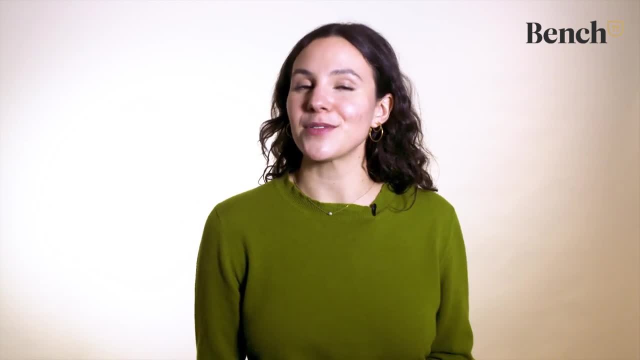 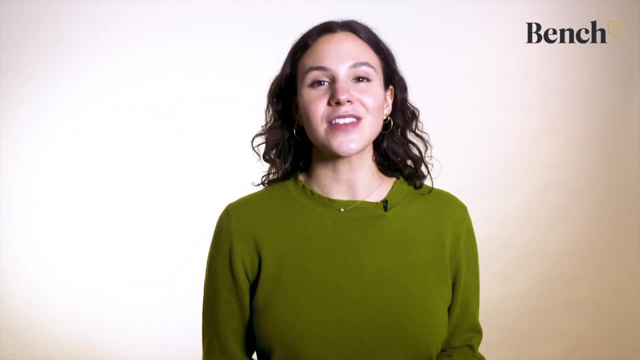 but your cash flow statement says that you only made $5,000 in cash. What's going on? Well, it could be that you sent out two invoices to clients for $5,000 each, If you're using the accrual system of accounting. 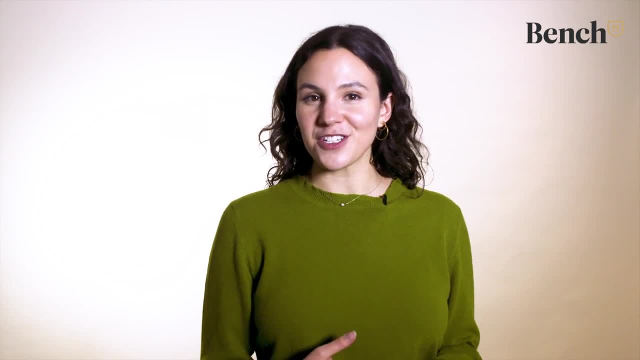 you would record that $10,000 as revenue in March, even though you haven't gotten paid yet. Then one client pays you, but the other client is late. Your income statement would say $10,000, but your cash flow statement would say $5,000. 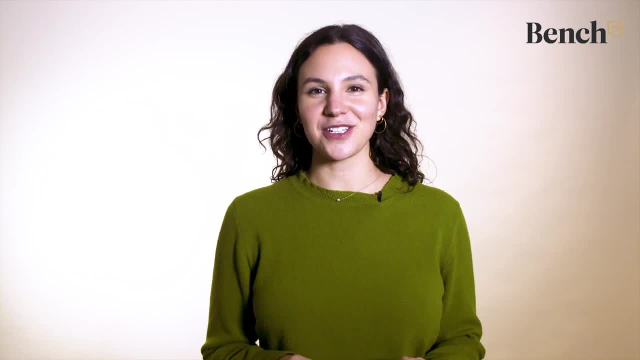 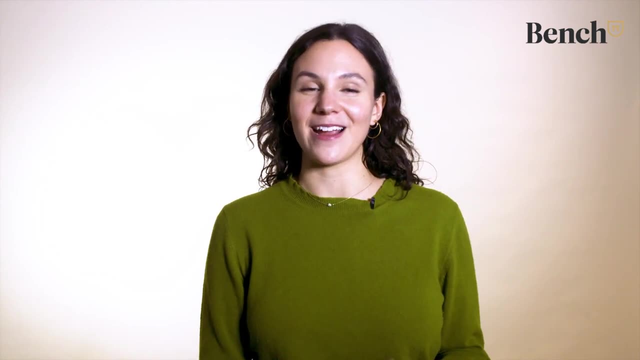 It's super important to know what the cash situation of your business is. If you don't have cash, you can't pay bills, even if you have accounts receivable money on the way to you. This is what a cash flow statement looks like. 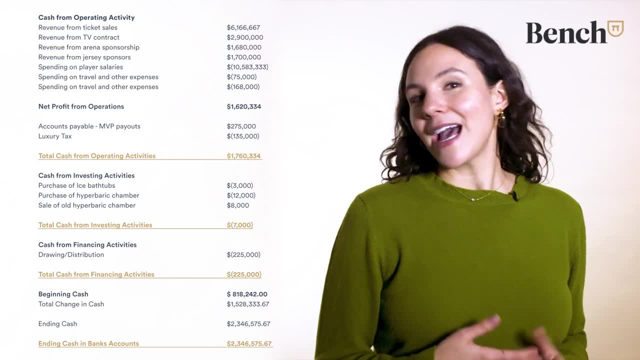 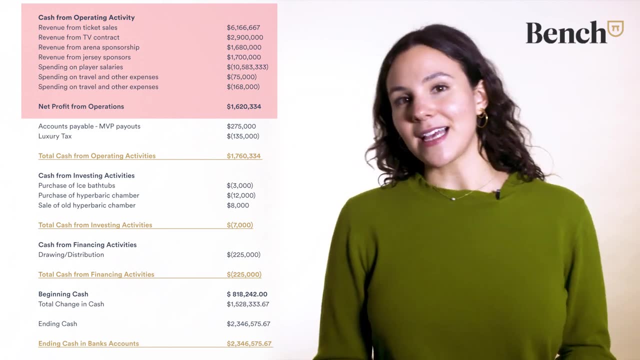 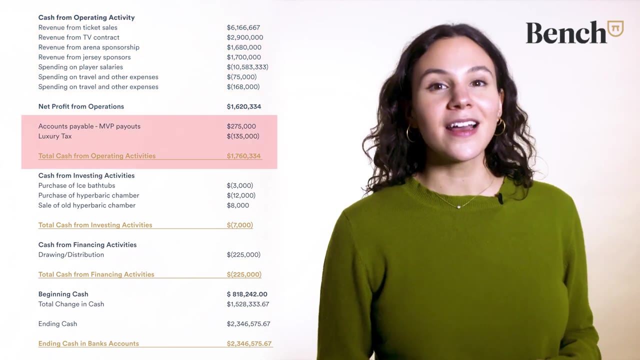 This is one from the Toronto Raptors. The cash flow statement has three parts. The first is cash from operating activity. This is all the core business activity: Buying stuff and selling stuff. Below that you see adjustments, things like accounts payable and luxury tax. 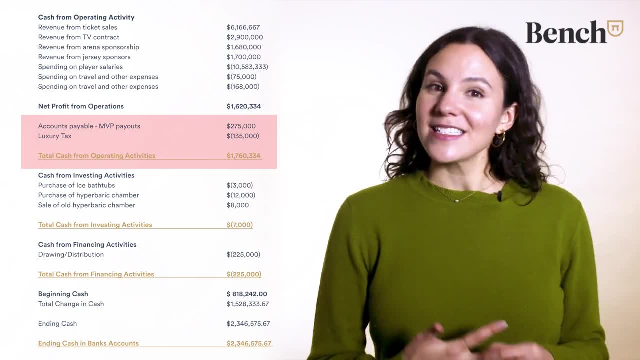 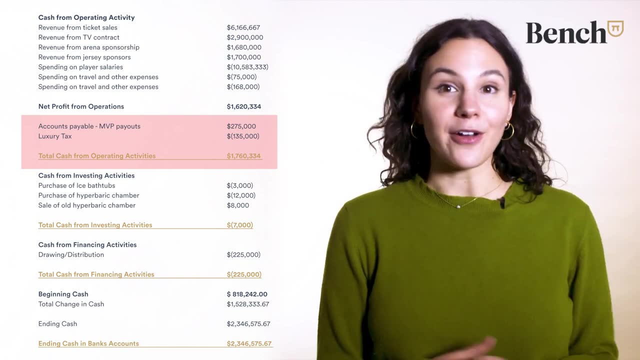 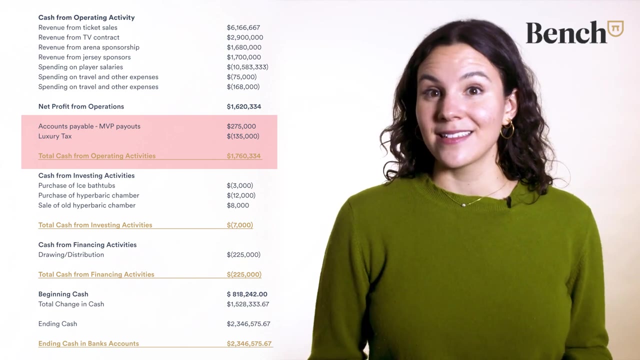 Taxes aren't from operating activity, but they still come out of our cash, so we subtract it. Accounts payable technically isn't a cash transaction at all. However, on the income statement it's marked as an expense, even though it's money that hasn't been paid out yet. 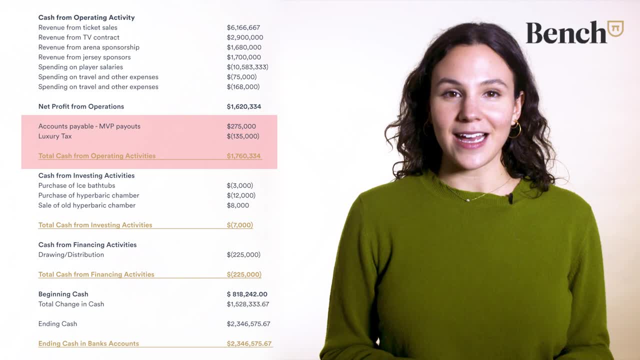 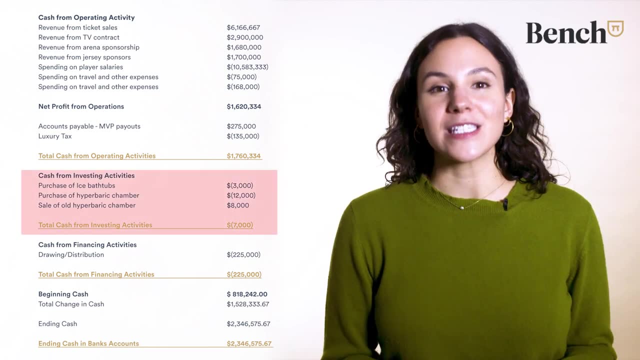 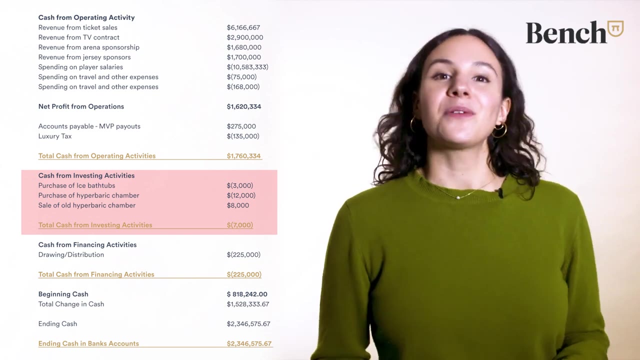 So we add it back into the cash flow statement so we get an accurate picture of how much cash we actually have today. Next is cash flow from investments in your business, So not the regular buying and selling of your core business, but things like equipment, work, vehicles, etc. 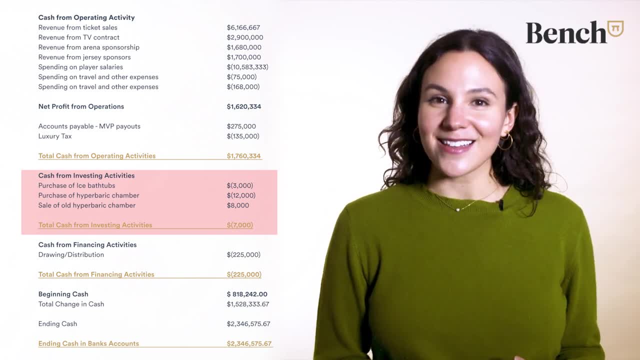 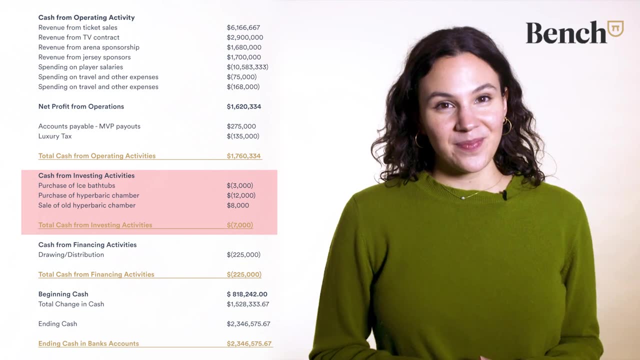 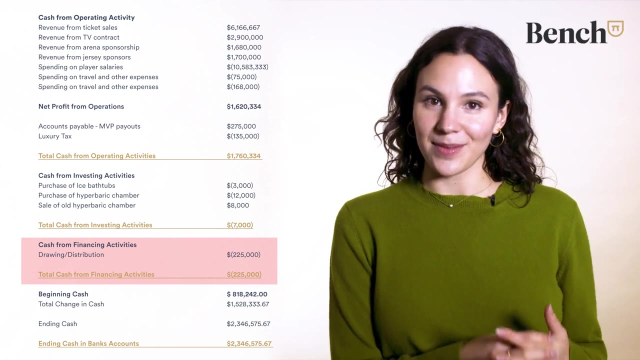 In the case of the Toronto Raptors. here they bought an ice bathtub and a hyperbaric chamber for athletes to recover after games, And they also sold a hyperbaric chamber. The last category is cash from financing activities. This includes money the owner invested in the business. 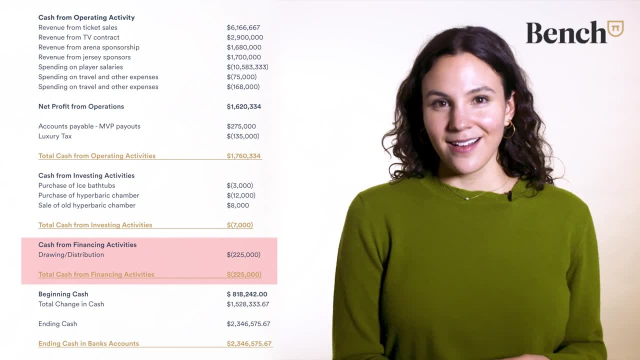 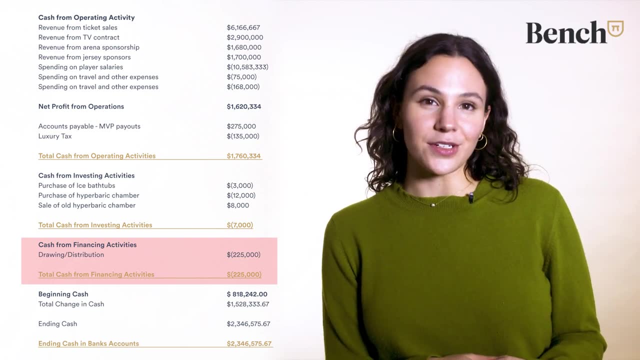 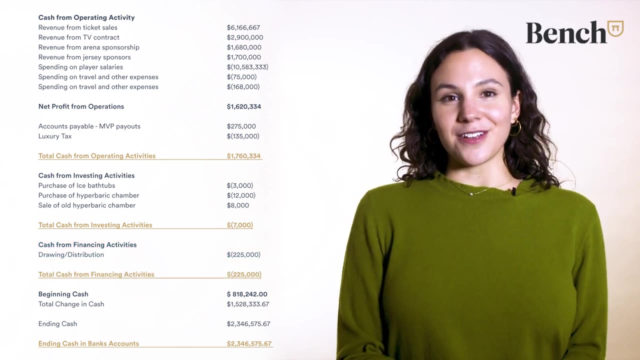 as well as taking out and repaying loans. On the Raptors statement, we see there was an owner's draw, which means the owners withdrew $225,000 from the business. This basically means they paid themselves If you add all three categories together. 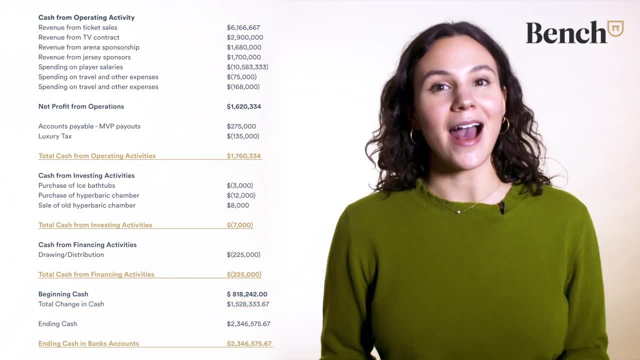 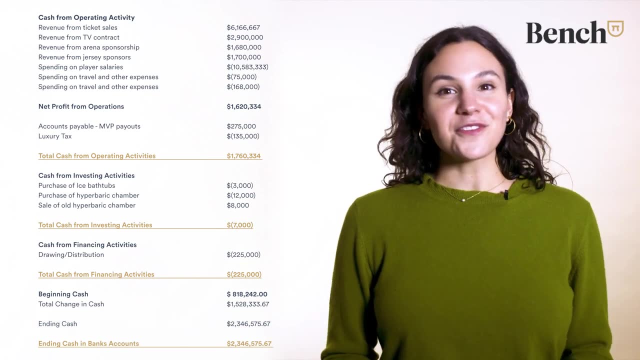 you get the total change in cash. If you add the beginning cash to the total change in cash, you get the ending cash And for good measure you check your ending cash against what your bank account actually says to make sure you added everything up correctly. 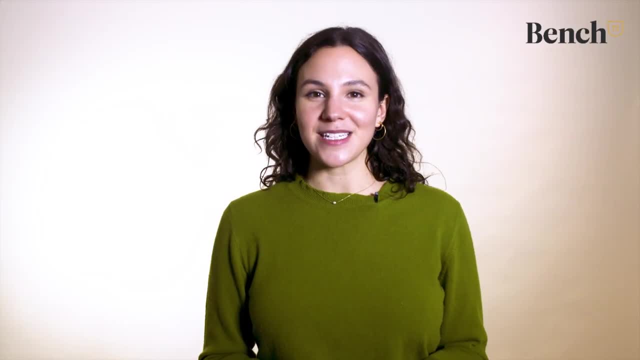 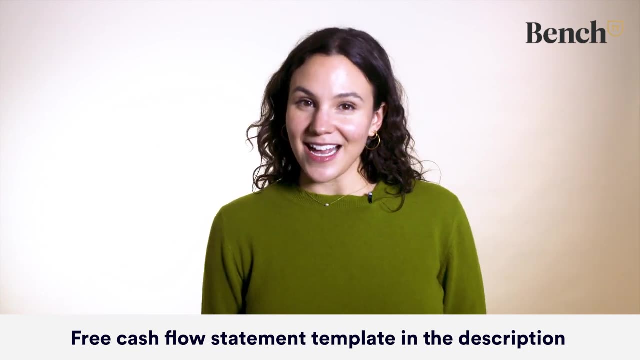 If you want to create your own cash flow statement, you can download our template in the description below. Just plug in your numbers and you have a basic statement you can use to analyze your cash situation today. That's the end of our Financial Statements- Crash Course. 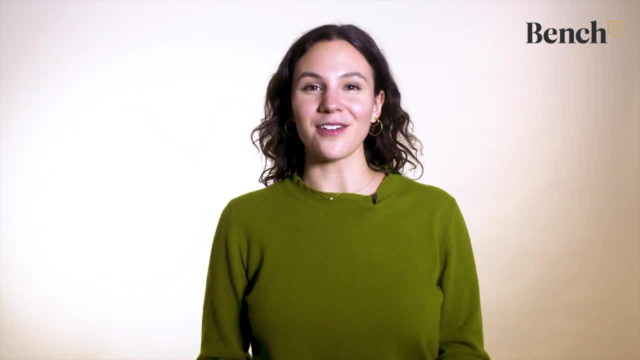 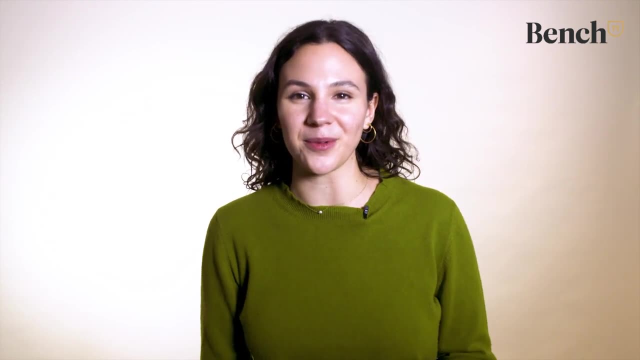 If you're an accounting pro using accounting software, you can create these statements today. If you're less comfortable with accounting, you're probably going to want to hire a bookkeeper to do it for you If you don't have a bookkeeper today. 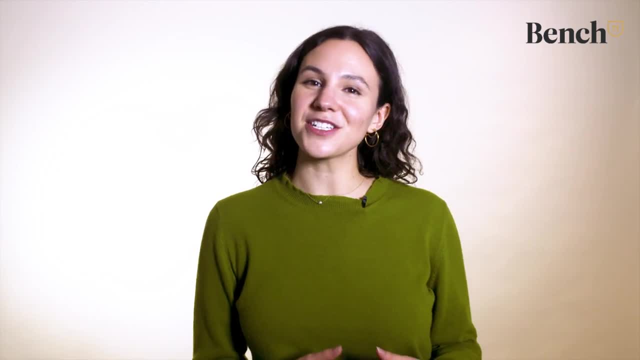 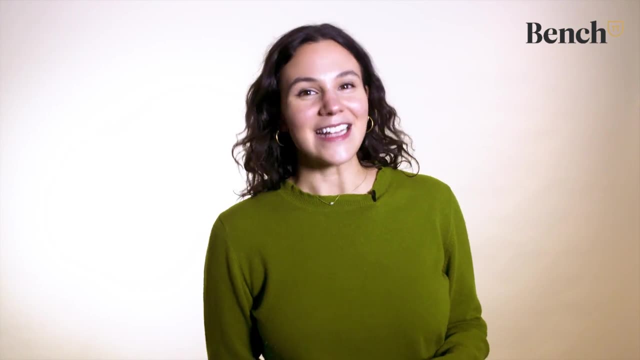 check out Bench. We'll do your bookkeeping for you and send you financial statements every month so you can make smart business decisions and stay on top of your finances. That's it from us here at Bench. Good luck on your entrepreneurial journey and happy bookkeeping. 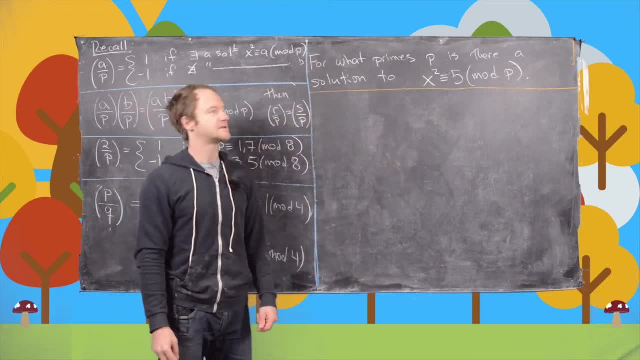 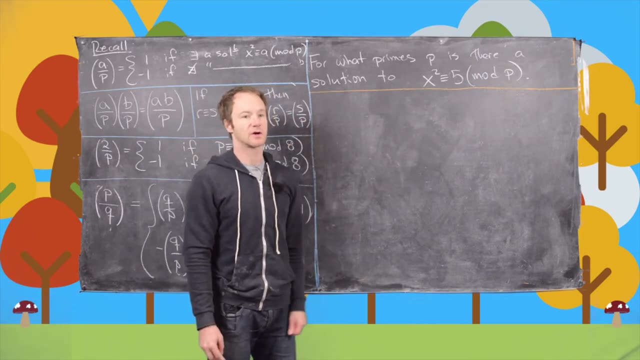 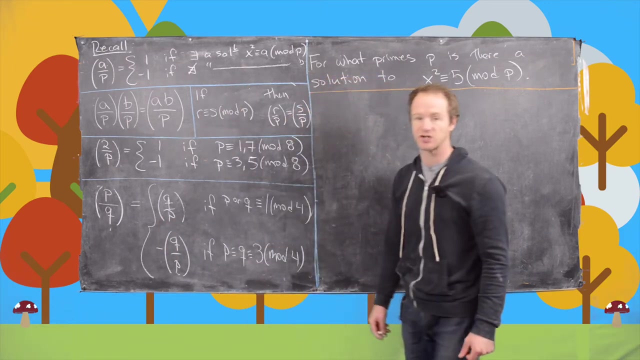 In this video we're going to answer this question. So, for what primes p is there a solution to this quadratic congruence? x squared is congruent to 5 mod p. In other words, for what primes p is there a square root of 5.? Okay, good, we're going to make use of the Legendre symbol and